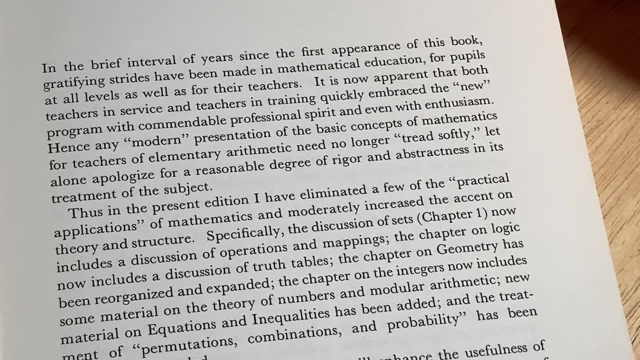 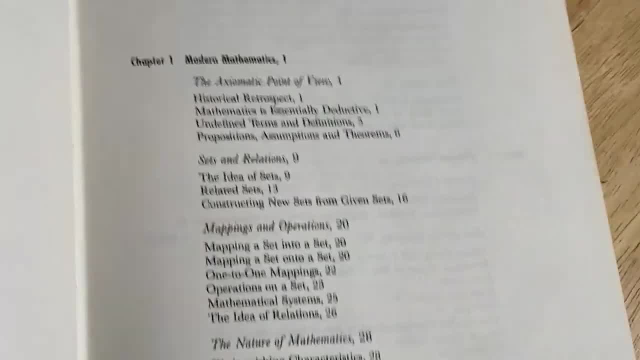 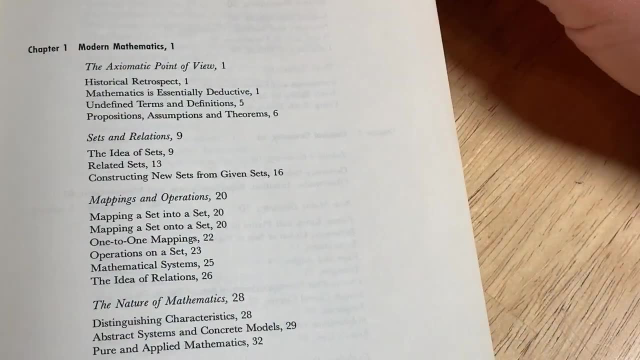 pupils at all levels, as well as their teachers. Okay, So this should just have really, really basic mathematics in it. Let's look. I mean, it is called Basic Concepts of Elementary Mathematics, So let's see what we got here in this textbook. So modern mathematics talks about sets and stuff. 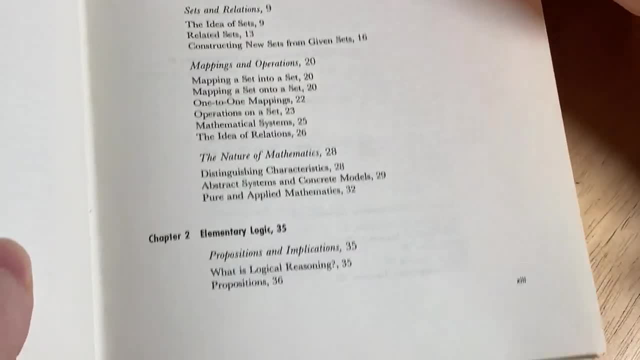 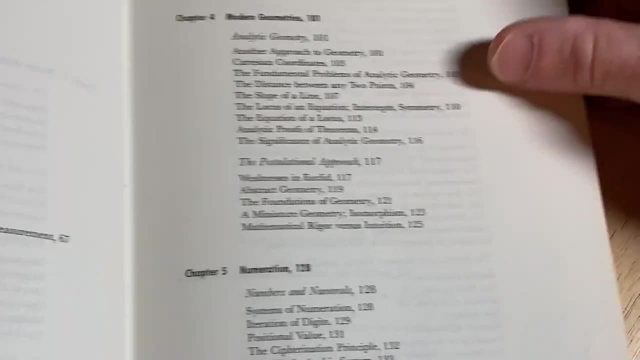 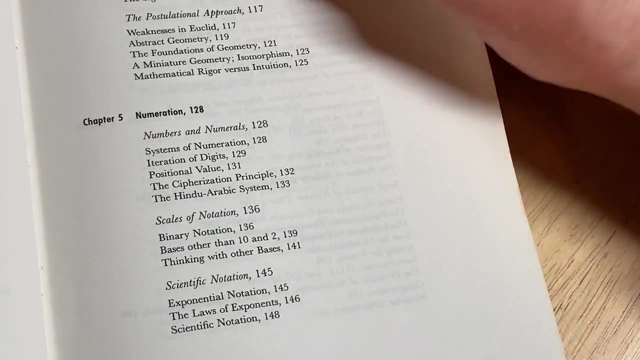 That's really important, Very important Logic. So you get some logic, reasoning stuff. Geometry: It's kind of like a finite math book in some sense. It has just like a bunch of different topics: Modern geometries, Numeration talks about the different number systems. Yeah, 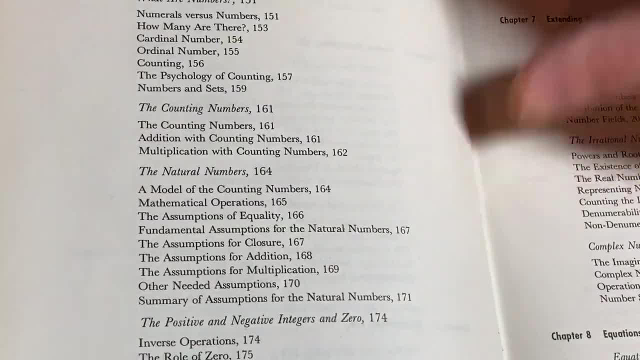 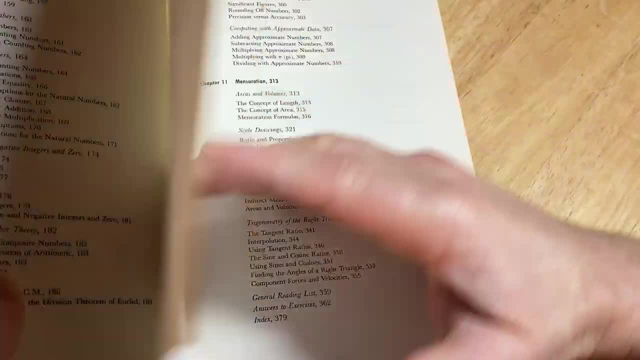 this is typically stuff you would see in like a finite math book: The number concept Extending the number system. Then you have equations, inequalities and functions, Just like a survey of math right Permutations. You get some counting Some. 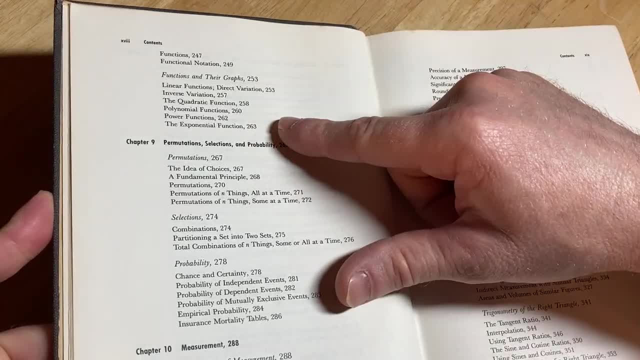 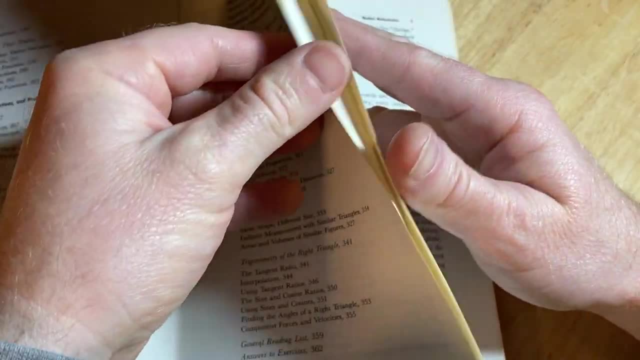 measurement. Here you get quadratic functions, polynomials, exponentials, So you're introduced to a lot of different areas, A lot of different types of mathematics in this book, And that's it. And there's a quote here with the quote saying: mathematics is the science that uses easy words. 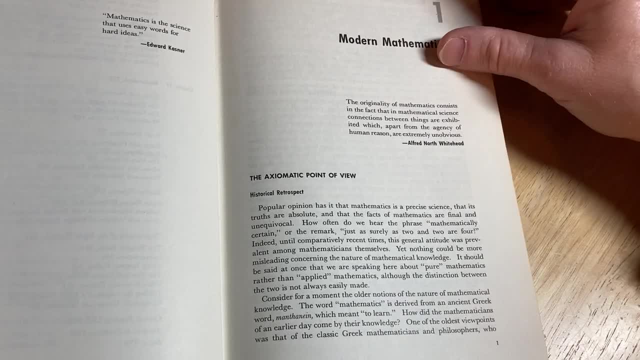 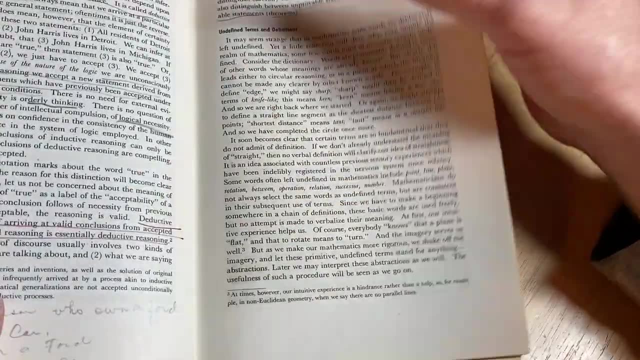 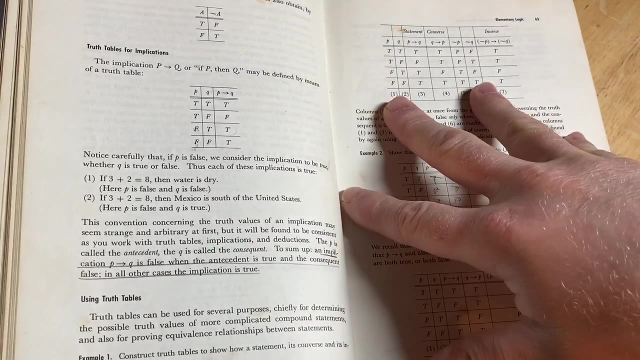 for hard ideas. Yes, Yeah, modern mathematics, The axiomatic point of view. So you get some reading here And then you have some exercises. Here's some truth tables. This is something you do in a discrete math course or in a logic improved course or sometimes in a finite math course, So something that you see a. 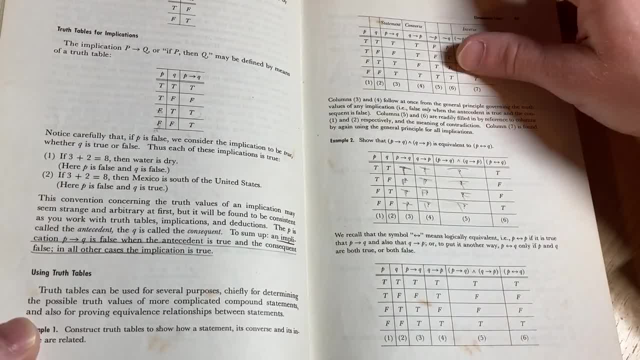 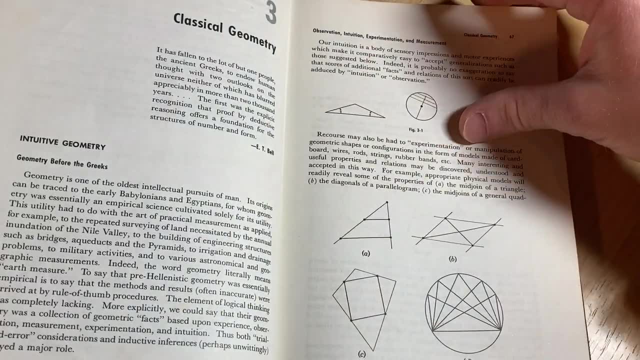 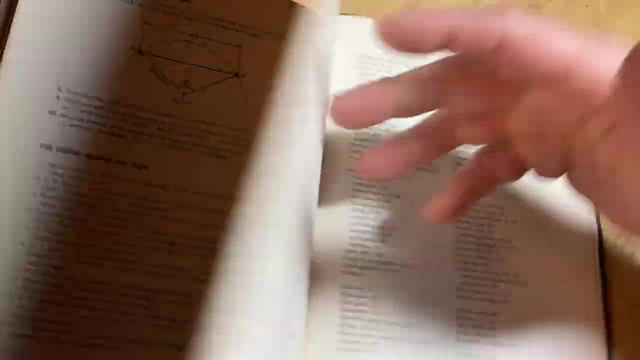 lot of is truth tables And that's pretty cool to read in this book. Learn some truth tables. They give you some references here for further reading and study Geometry. So it's just a book that kind of has like a survey of different areas of math. 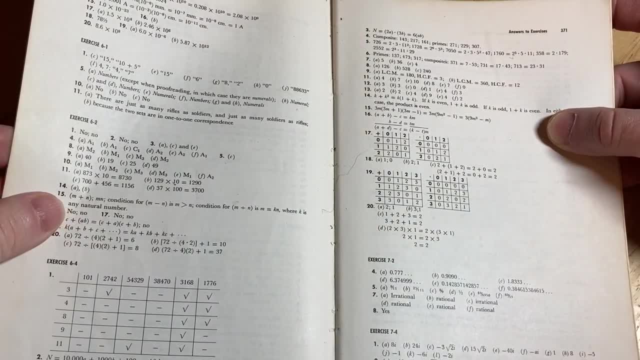 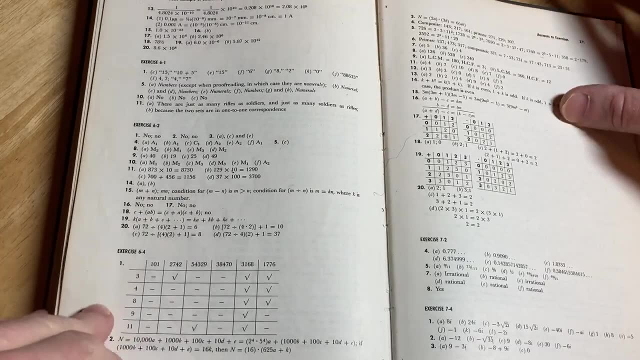 And then here we have some answers to the exercises in the back of the book. You don't have all of them. It looks like you don't like five And then you're missing six and seven, But you do have quite a bit, which is really good. Not everything, but it's better than nothing.